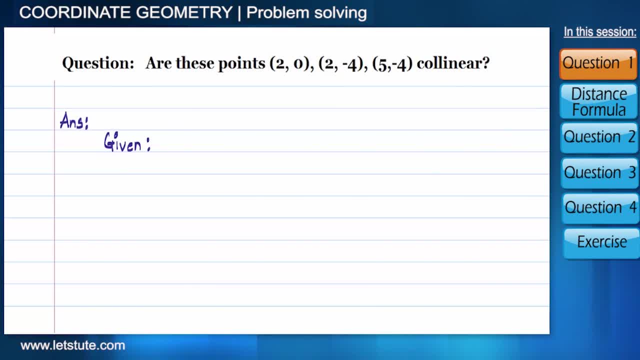 So here we proceed. The given part is 3 points, So let's name them Now. these points are P, Q and R, And we have to see whether points are collinear or not. So this is the tool which will help us to find the distances between the coordinate. 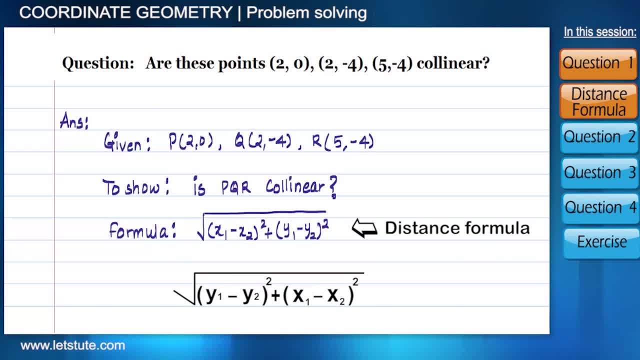 points. Friends, you can write this in such manner. Now let me change the way of writing two points, That is, by adding the square root of 2 to 2x2y1 and电지 수2y2y2, or P and Q. 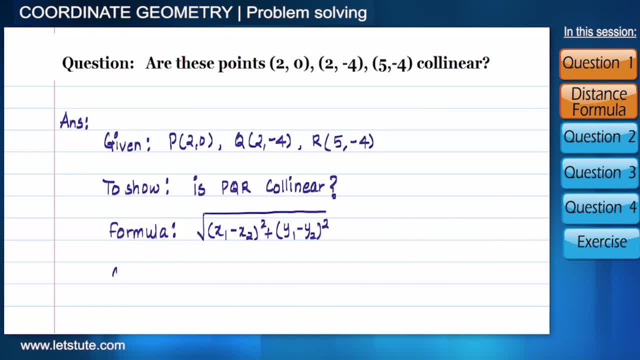 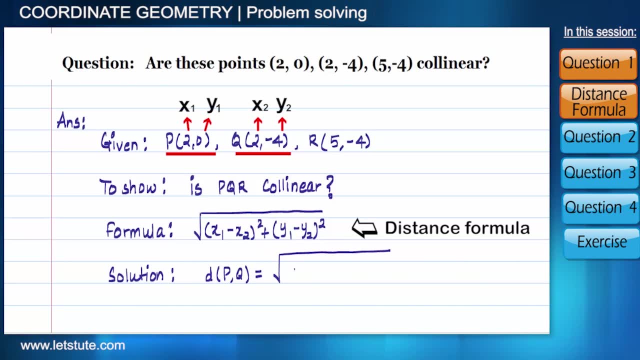 Now add two points in x and y. well, Let's add z and z and y as well, And we have solved this problem fine. Now we'll try to solve it in such manner as well. Order of x1,, x2, and 1,y2 doesn't matter. 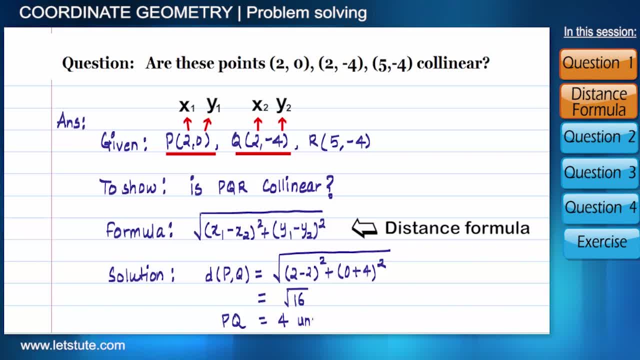 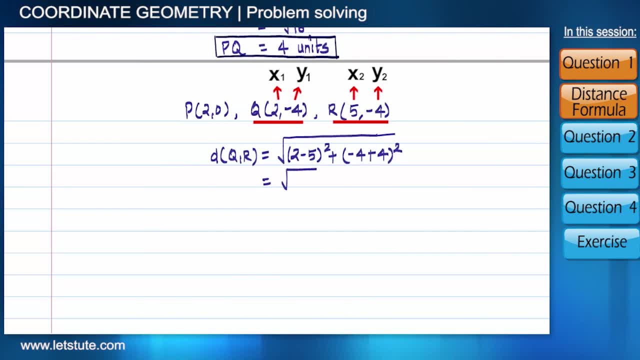 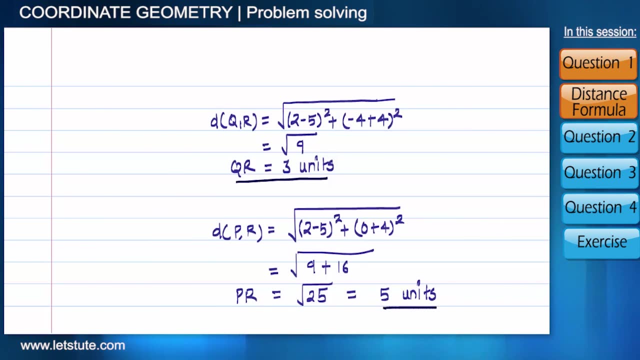 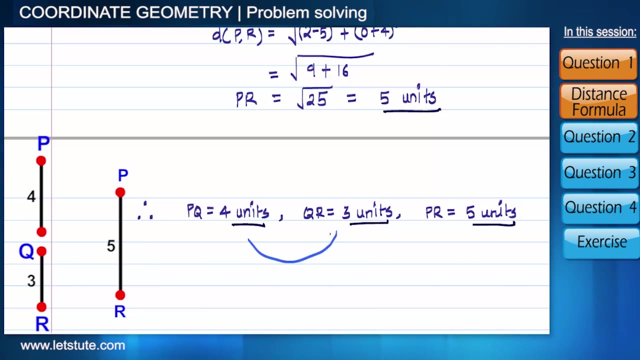 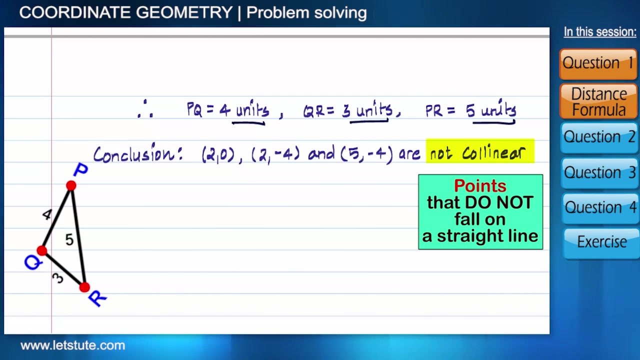 which comes out to be this much distance between QR and distance between PR. I found the distances and noticed that addition of these two small numbers is not equal to the remaining bigger one. So I conclude that they are not collinear Friends. you can say that before starting the solution. 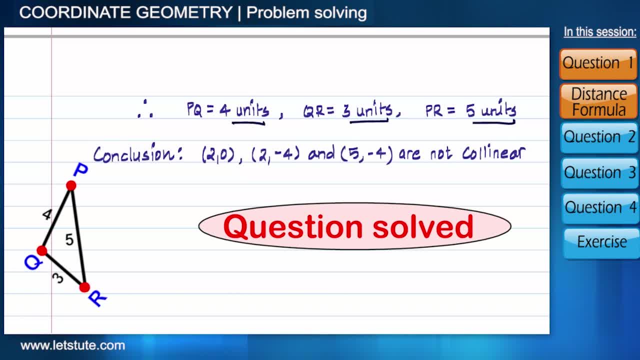 we discussed a lot and after that we solved it quickly, without any mistake. But, as we discussed, if points are not collinear, they will form a triangle. So, friends, can you tell me what kind of triangle it is? We recognize the types of triangles by looking at their sides. 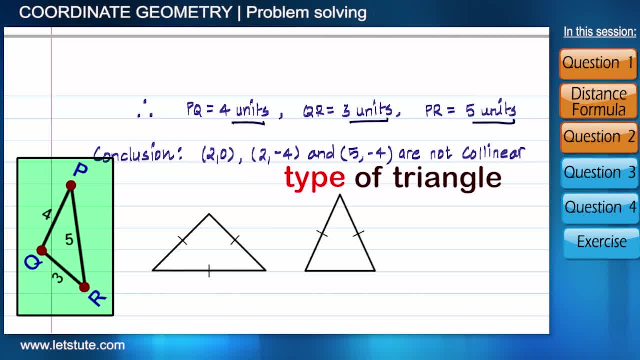 whether all of the sides are equal, only two sides are equal or all of them are of different lengths. So if all the distances are equal, it's an equilateral triangle. If only two distances are equal, then it's an isosceles triangle. And the third case is: 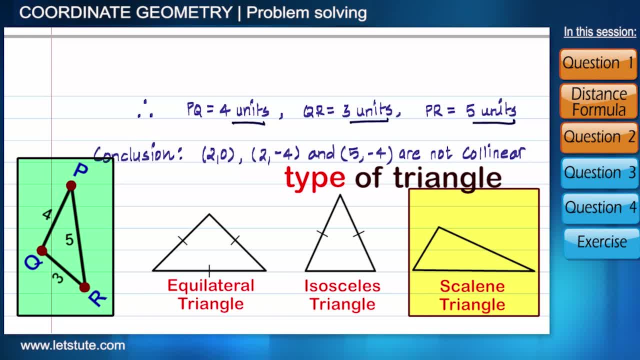 the triangle may be a scalene triangle as well. In our case, all the sides are of different lengths, So it is neither equilateral nor isosceles. That means it's a scalene triangle. Friends, a triangle may be a right angled triangle also. So if we want to check whether our triangle 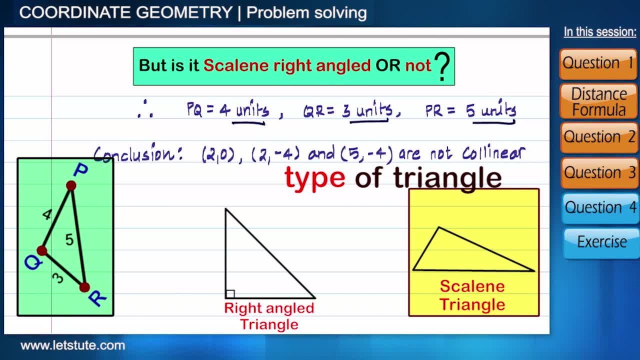 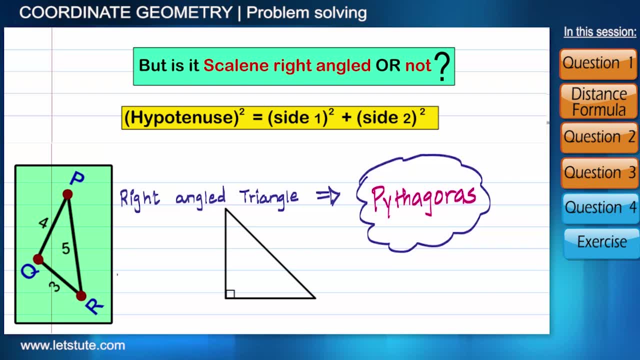 is right angled or not. For that, what must we do? As we hear the name right angled triangle, suddenly Pythagoras theorem pops up in our mind. So square all the values and see if sum of any two small numbers is equal to the remaining bigger one or not. 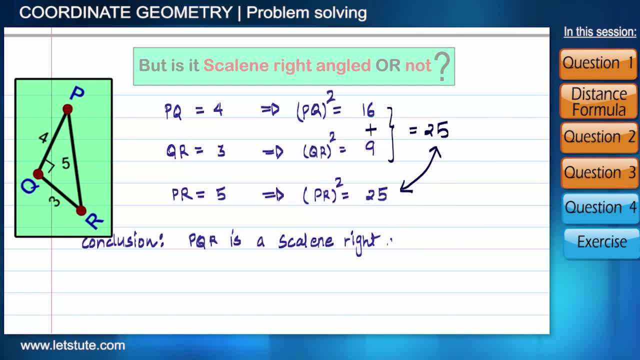 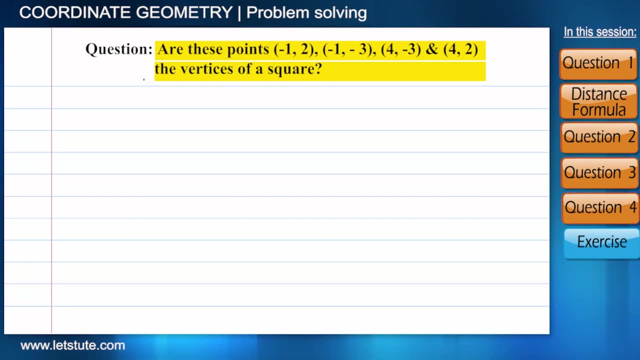 So I found that it's a scalene, right angled triangle. See how easily things are. We just need to concentrate a bit and apply a little bit of logic. Alright, Let's quickly have a look at this question. Are these points the vertices of a square? Let me tell you the idea behind it. 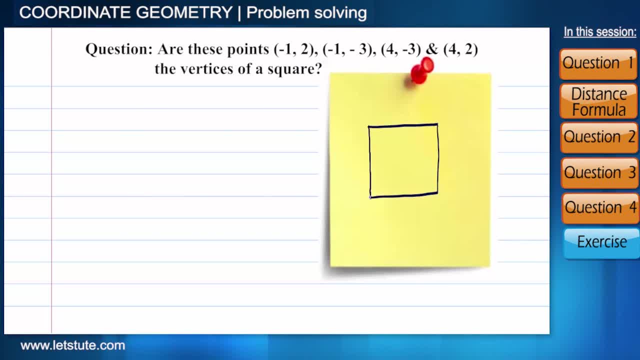 First of all, I'll make an imaginary diagram of a quadrilateral ABCD. Now, If AB, BC, CD and AD are equal means it's a square Right, So we'll find all the distances, But still this is not the whole solution, Even if all four distances are equal. 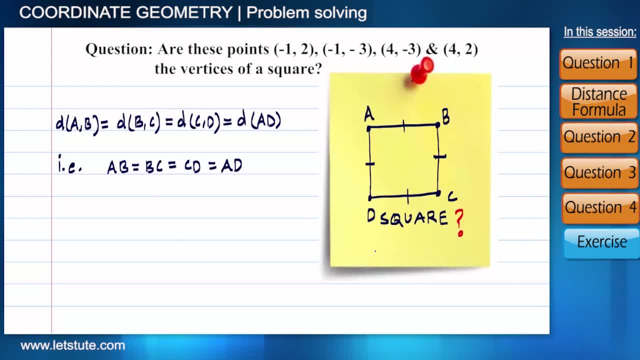 We cannot say that it's a square, Because it may be a rhombus as well. Now what to do? Another property of square is that its diagonals are also equal. Therefore, with all four sides, we'll also have to find whether diagonals AC and BD are equal or not. 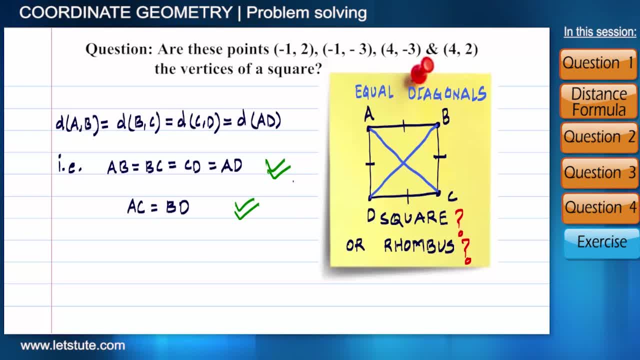 Now this will be the proper solution. You must be thinking: If we directly find AC and BD, the lengths of the diagonals, Is it enough to check for a square? The answer is no, Because even rectangle and isosceles, trapezium also have equal diagonals.